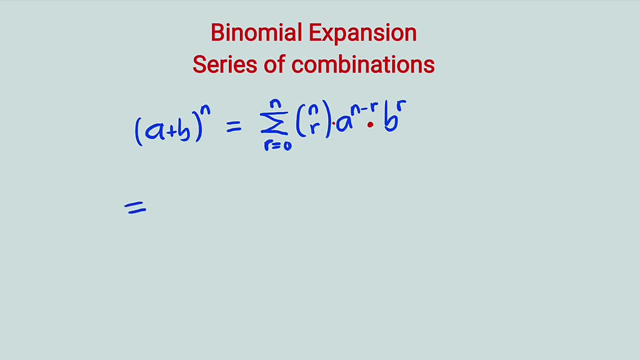 In order to take this series, we are going to be increasing the value of r from 0 down to n. As soon as the same goes to n, we stop. This is equal to n combination 0 when r is equal to 0.. 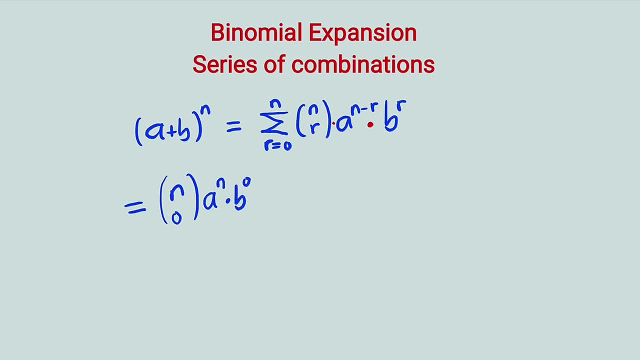 b raised to the power of 0, which is the same thing as 1.. Then, plus you increase the value of r, We have n combination 1,, a raised to the power of n minus 1, then b raised to the power of 1.. 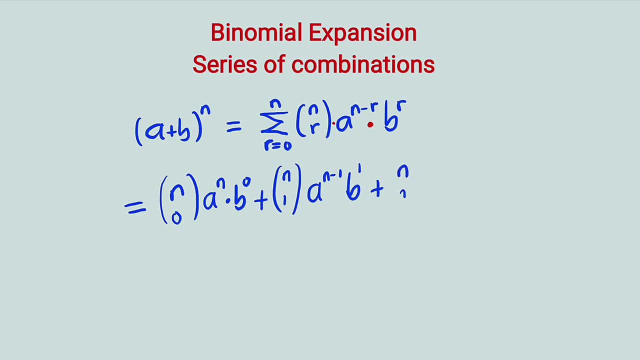 You add n combination 2, a raised to the power of n minus 2.. b raised to the power of 2.. This is how you keep on going till you reach the last term, which is n combination n, As r is equal to n. a raised to the power of n minus n, then b raised to the power of n. 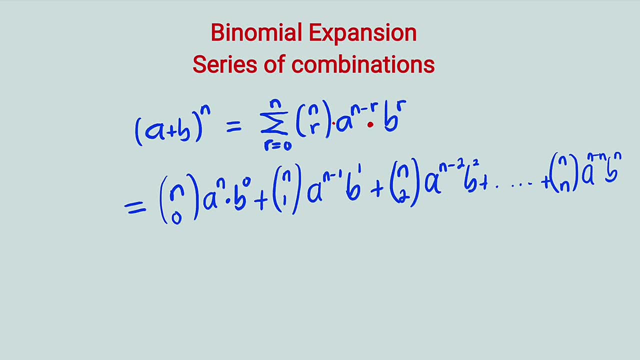 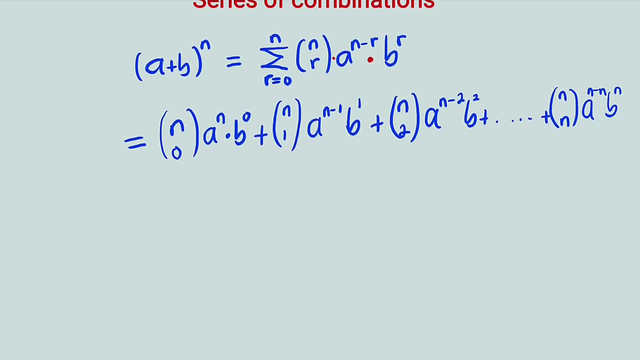 You know, n minus n will be 0, so in the last term, a will be to the power of 0, which is the same thing as 1.. And one thing you should know is that n combination r can also be written as n combination r. 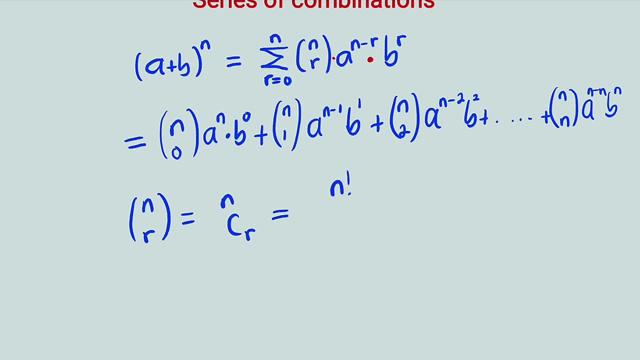 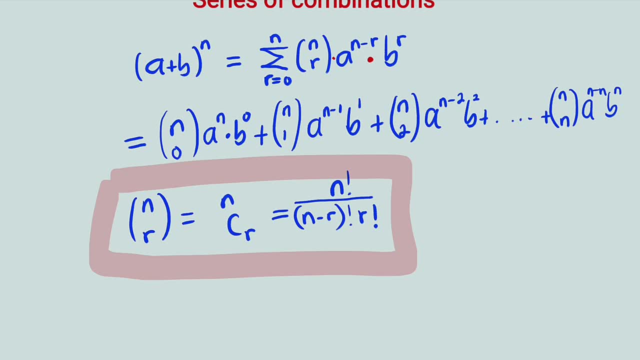 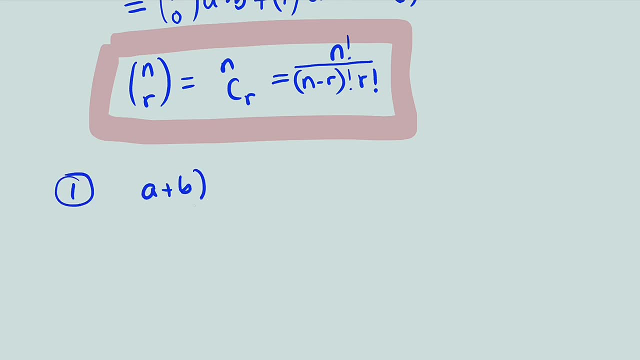 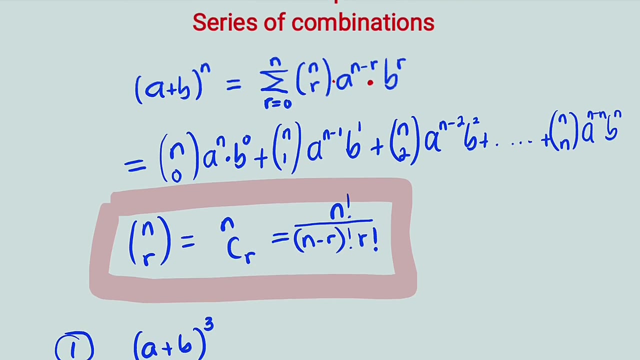 So now let us take a look at the definition of combination. let us take some problems at random like 2 or 3.. Number one: suppose we want to expand a plus b raised to the power of 3, for example, where our n is equal to 3 in this case. So 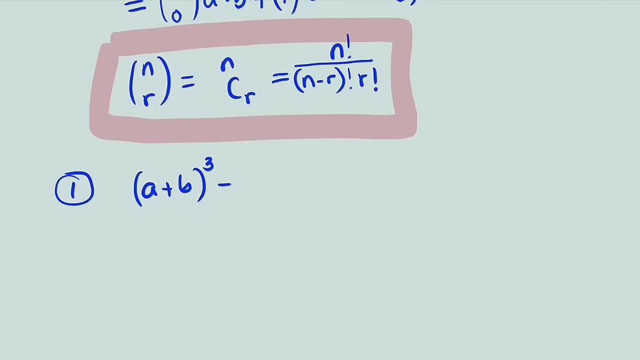 we have only four times. So this is equal to 3 combination 0. That's the first time when r is equal to 0.. a raised to the power of n minus 0, then b raised to the power of 0 plus 3 combination 1, a raised to the power of n minus 1, that is 3 minus 1 equal to 2,. 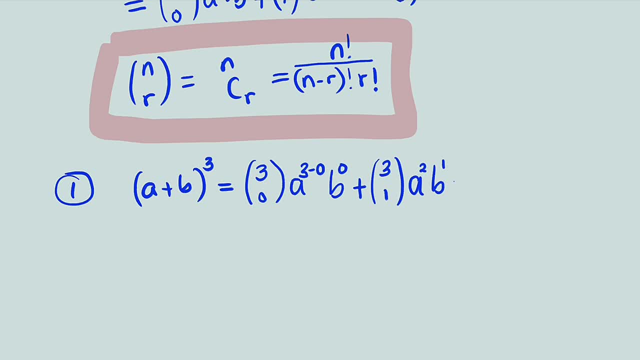 then b raised to the power of 1 plus 3 combination, 2, a raised to the power of n minus 2,, that is, 3 minus 2, which is equal to 1, then b raised to the power of 2.. And the last one, let me bring it down: 3 combination. 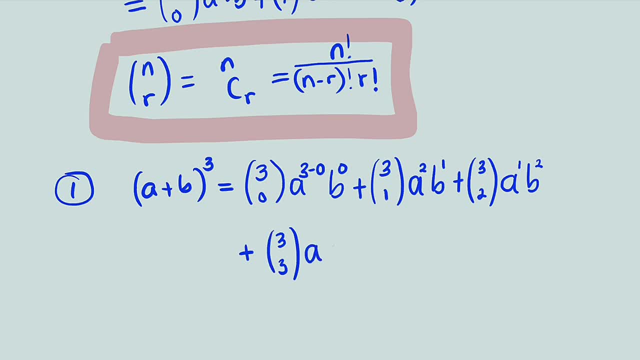 3, a raised to the power of n minus 3, that is, 3 minus 3 equal to 0, then b raised to the power of 3.. So one thing you should understand is that when you have a combination of three combinations, 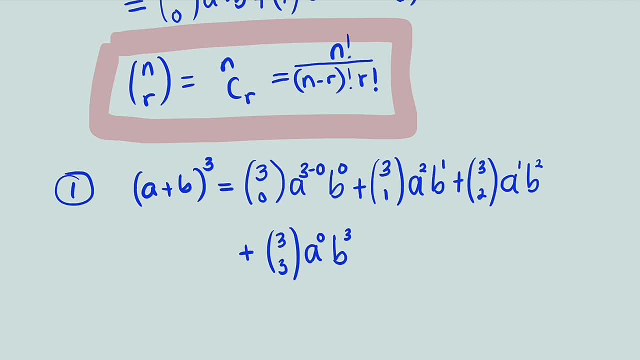 if you have direct Here you have a combination. So you would do: b raised to the power of 1 times 3, then you would do a combination of three combinations: 2 to the power of 1, but then you would say that b raised any one of the three combinations at the the dunno. So the combination is equal. 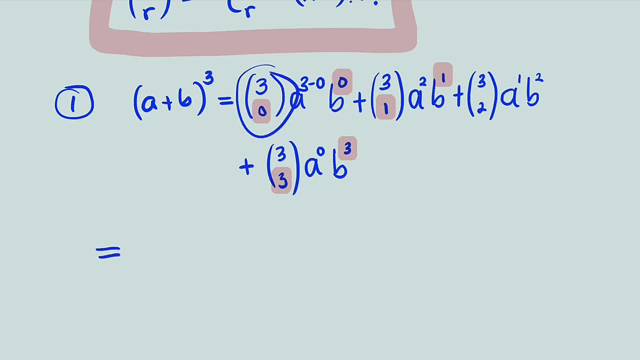 to different situation, as n raised is equal to 3xx first, and 1 raised is equal to 1.. So even in this case, if you have low hat characters, you may want to go out and read to say that 0 factorial, then 0 factorial, then we have a raised to the power of 3 minus 0, which 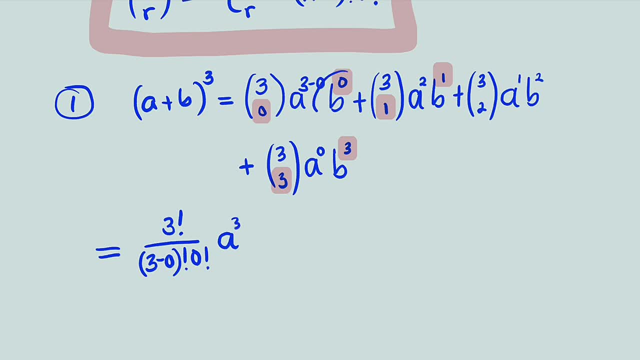 is the same thing as a raised to the power of 3, then b raised to the power of 0 is 1, so multiply by 1.. You take the next term, 3, combination. 1 is the same thing as 3- factorial. 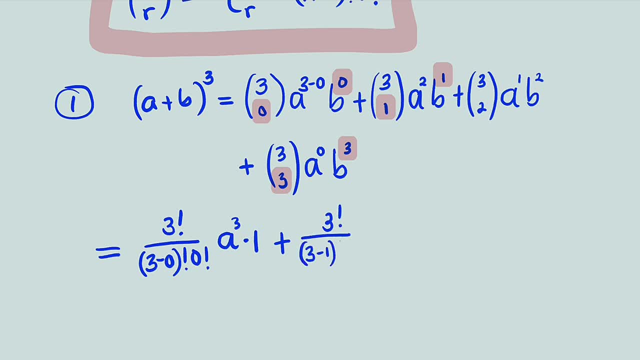 divided by 3 minus 1 factorial, then 1 factorial, then a has a power of 2, b has a power of 1.. You don't even have to write power of 1.. Plus 3 combination 2 is the same thing as 3. 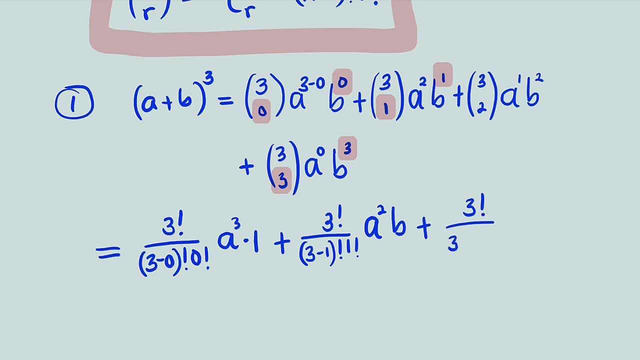 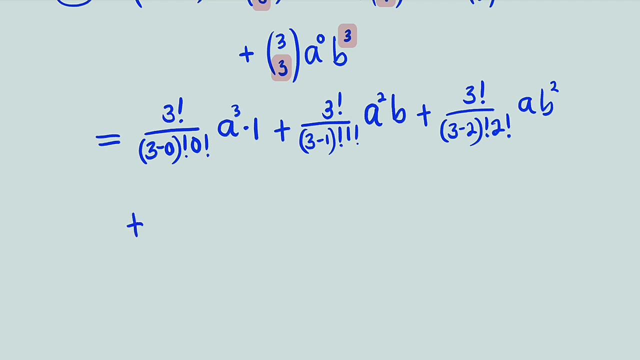 factorial divided by 3 minus 2 factorial, then 2 factorial. a has a power of 1.. b has a power of 2.. Then the last term, 3 combination 3, that is 3 factorial divided by 3 minus 3 factorial. 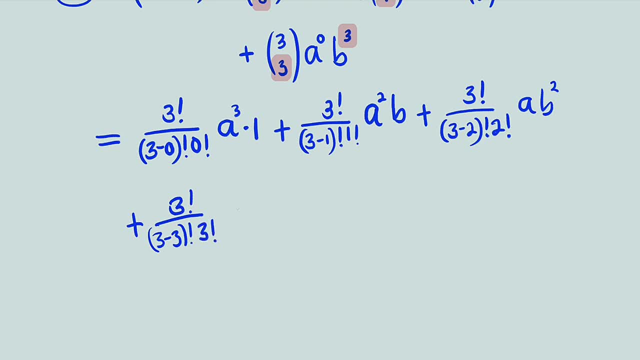 then 3 factorial. a has a power of 0, so it becomes 1, and b has a power of 3.. So the next thing to do here is to simplify And remember that 0 factorial is equal to 1 factorial, and all of them are equal to 1.. 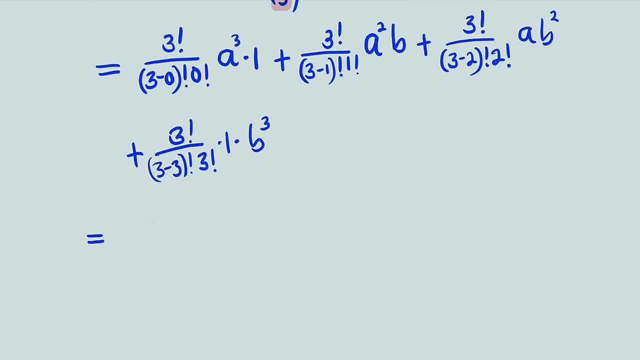 So let's begin. This is equal to 3 factorial to the top, divided by 3 minus 0 factorial is 3 factorial, then 0 factorial, We have a to the power of 3 times 1 is still a to the power of 3,. 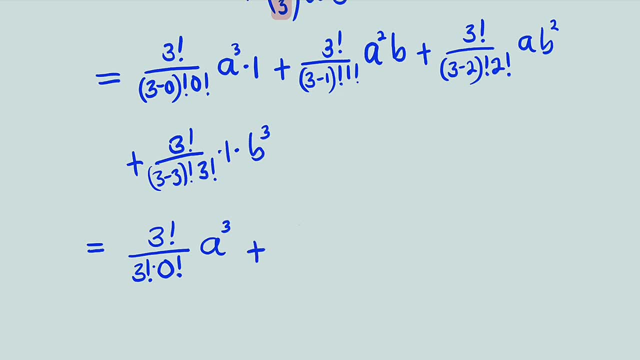 then plus We have 3 factorial to the top, divided by 3 minus 1 is 2 factorial. then, multiplied by 1 factorial a to the power of 2, b to the power of 1, plus 3 factorial divided by 3 minus 2 is 1 factorial multiplied by 2 factorial. 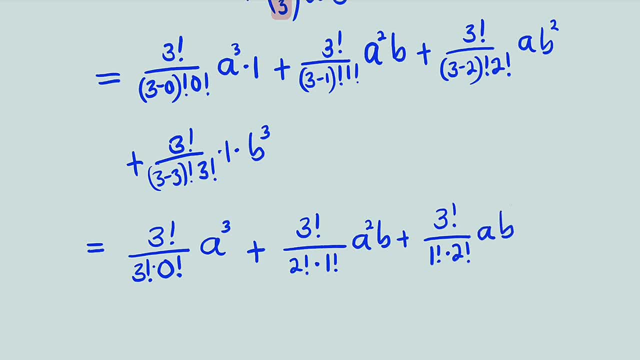 a with power of 1.. b with power of 2 plus the last one, 3 factorial. 3 minus 3 is 0 factorial. then 3 factorial 1 times b to the power of 3 is b to the power of 3. let's further simplify this. 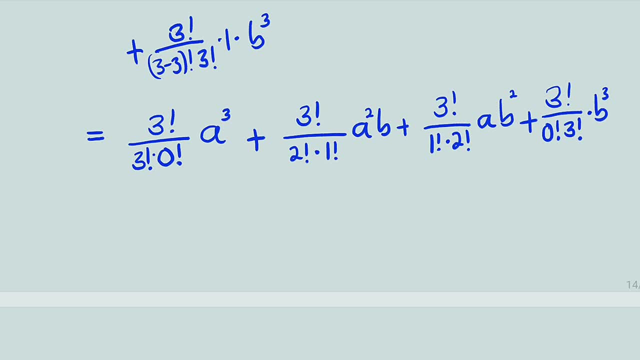 we can cancel something here because 3 can cancel 3. i remember that 0 factorial is equal to 1. so from the first term we only have a to the power of 3 plus the second term. the second term, we have 3 factorial divided by 2 factorial. remember, 3 factorial is the same thing. 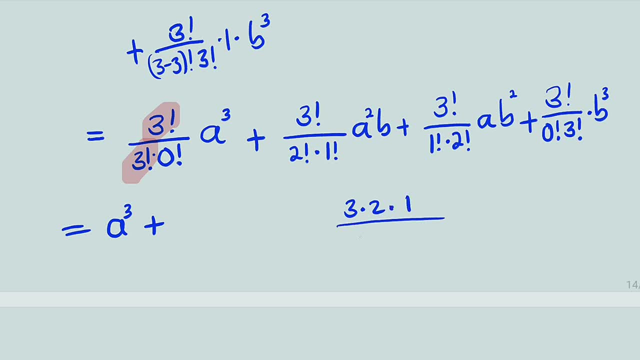 as 3 times 2 times 1, and 2 factorial is the same thing as 2 times 1. 1 factorial is also 1, so you can see that 2 times 1 is 2 and 2 times 1 times 1 is 2. 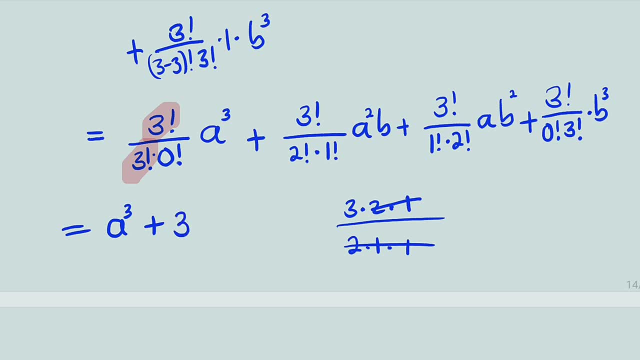 so we have only 3 there. so we have 3 a squared b. then, moving on to the third term, which is this, we have 3 factorial divided by 1 factorial times 2 factorial. look at the coefficient: they are exactly the same. so we have 3 a. b to the second power. 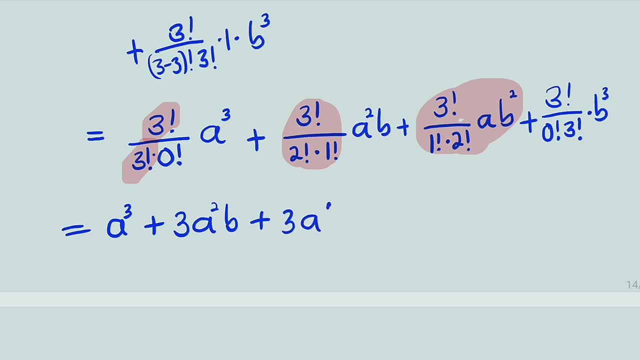 3, a, b to the second power, then the last one we have: 0 factorial is the same thing as 1, so this 3 factorial will cancel 3 factorial. what we have is only b to the power of 3, so we have b to the power of 3. 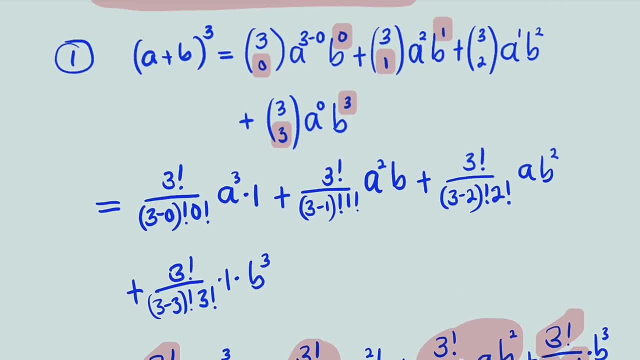 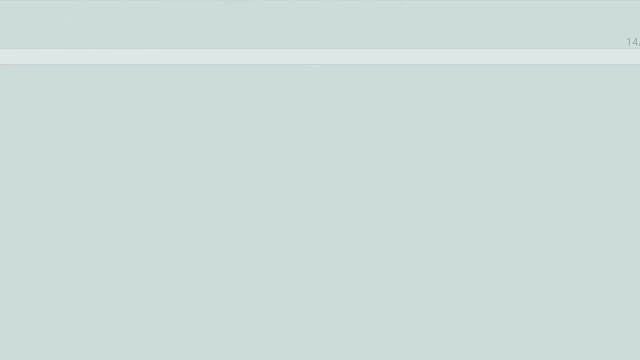 so this is just the expansion of a plus b raised to the power of 3, using combinations. now let us take another question. For example, suppose we wish to expand 2x plus 3 raised to the power of 4.. Let me come down here. 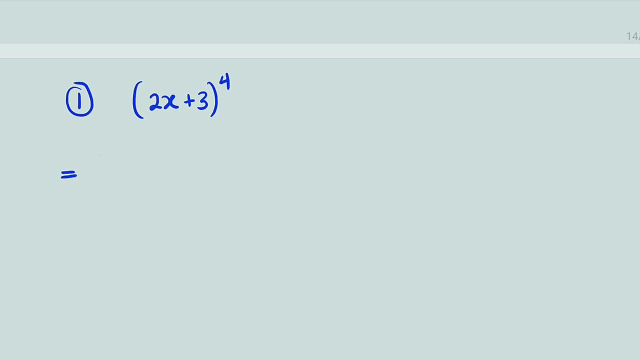 This is equal to n is 4 here, So we have 4 combination 0.. Our a is 2x, So we have 2x to the power of n minus 0.. 4 minus 0 is 4.. So multiply by b is 3 to the power of 0.. 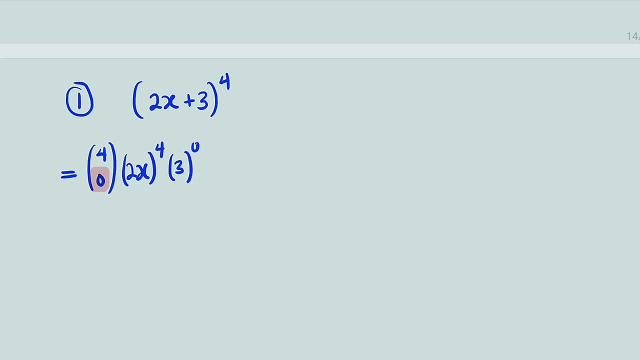 Because, remember I told you, the value of r will always be equivalent to the power of b. You take the second term, 4, combination 1.. a, which is 2x to the power of n minus 1.. That is, 4 minus 1 is 3.. 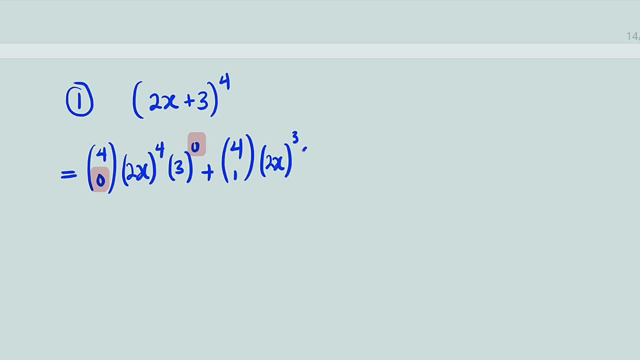 Then b will take that value of r, Which is 1.. So 3 raised to the power of 1. Plus 4, combination 2.. a, which is 2x raised to the power of n minus 2.. 4 minus 2 is 2.. 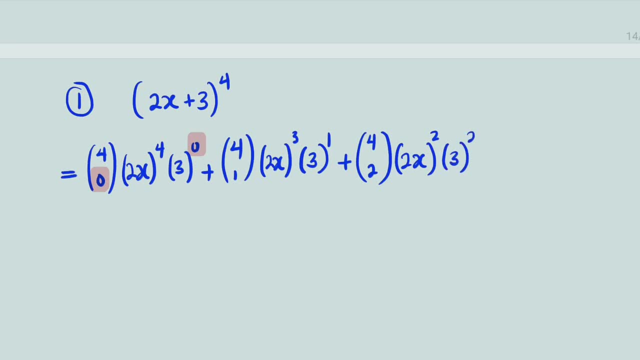 Then our b is 3 raised to the power of 2. Plus 4 combination 3.. a which is 2x To the power of n minus 3. That is 4 minus 3 is 1.. Then b, which is 3, raised to the power of 3.. 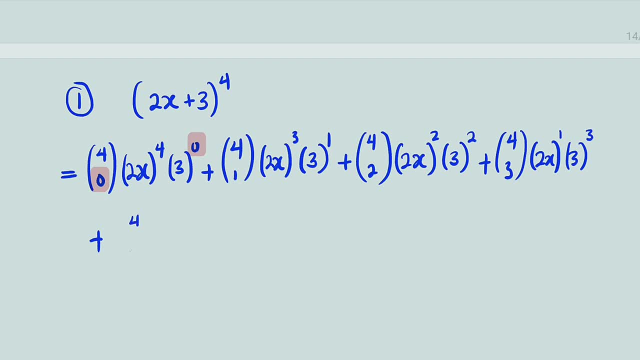 And the last term, we have 4 combination, 4.. 2x to the power of 4 minus 4 is 0. Then b, which is 3, to the power of 4.. So now let us simplify this. 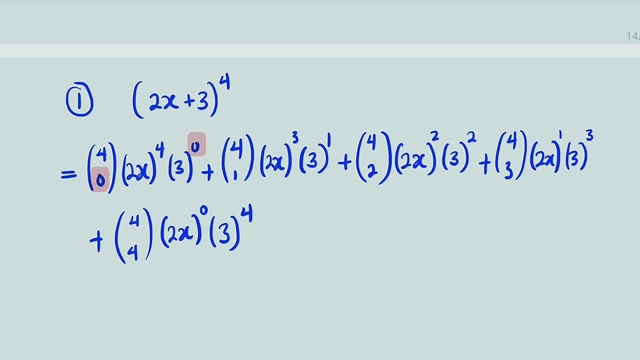 And there is something I wish to tell you: n combination 0. And n combination n are all equal to 1.. So if you simplify this, you have to get 1.. Likewise, this: 4 combination 0. And 4 combination 4 are all equal to 1.. 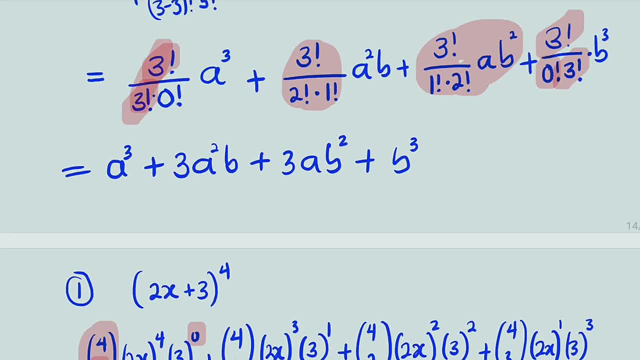 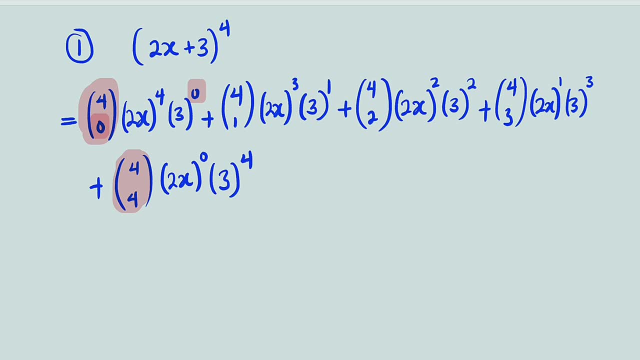 I have proven that for you. From here you can see This will cancel. And last one, you can see they will cancel. So we have no problem with 4 combination 0. We can just write the values 2x. 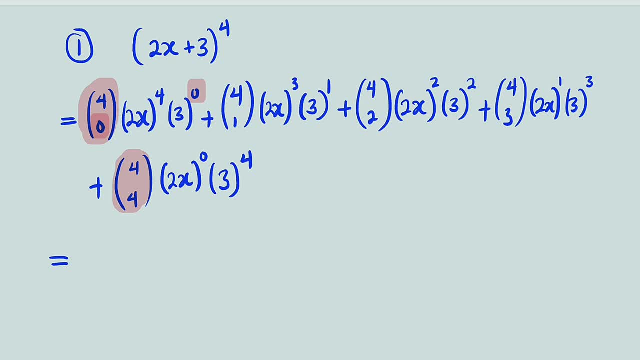 To the power of 4 will be 16x to the power of 4.. Already, 3 has a power of 0, which is the same thing as 1. So we have 16x to the power of 4.. Then we move to the second term. 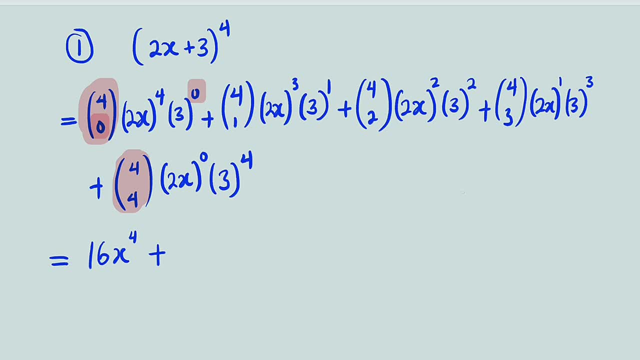 Let me simplify it to the other side. We have 4 combination 1, which is the same thing as 4 factorial. Divided by 4 minus 1 is 3.. So we have 3 factorial, Then 1 factorial. 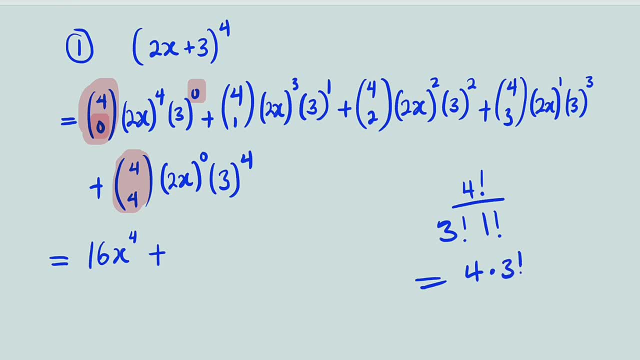 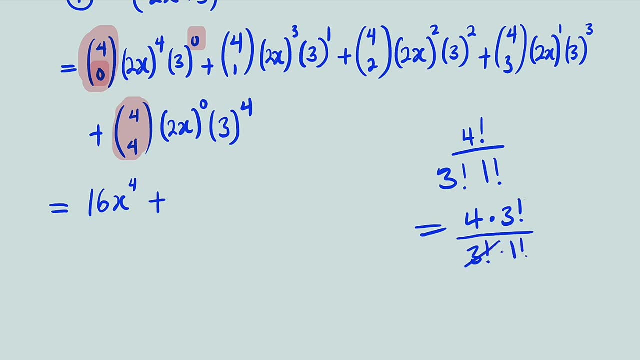 This is the Same thing as 4 multiplied by 3 factorial, Because I have 3 factorial to the bottom, So they will just cancel Times 1 factorial. This will cancel this Already. this is 1.. So we have 4 there. 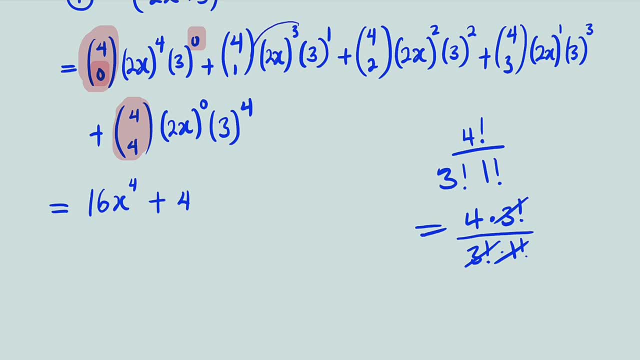 And that 4 will have to multiply 2x to the power of 3. Which is 8x multiplied by 8x to the power of 3.. Then multiply by 3 to the power of 1.. This is the same thing as 3.. 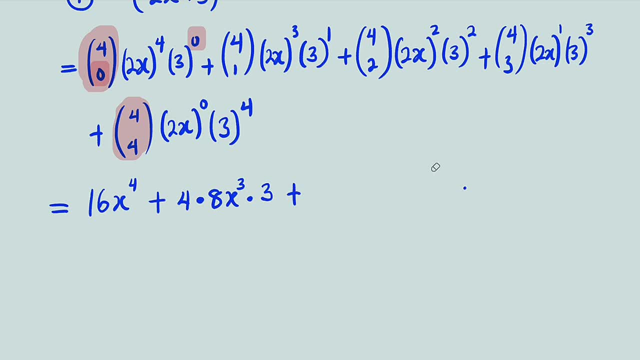 Plus 4 combination 2.. Let me simplify it here. It means 4 factorial divided by 4 minus 2, which is 2 factorial, Then 2 factorial. This is equal to 4, 3, 2 factorial. 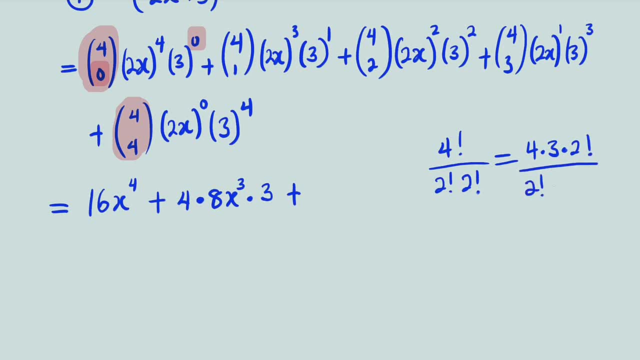 Because I have 2 factorial down here, 2 factorial And 2 factorial is 2.. This will cancel this And 2 can go into 4 two times. All we have is 2 times 3, which is 6.. 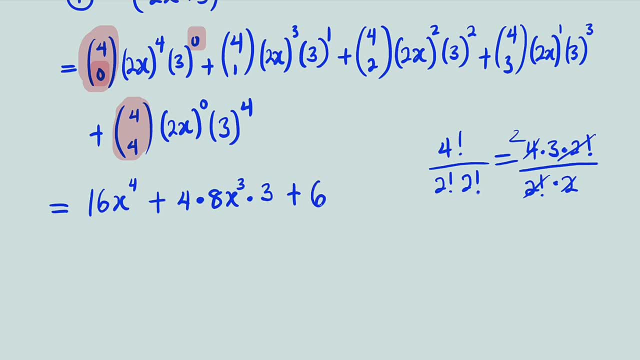 So 4 combination 2 is 6.. Then 2x to the power of 2 is going to give us 4x squared. Multiply by 4x squared, Then 3 squared is 9.. Then we move to 4 combination 3.. 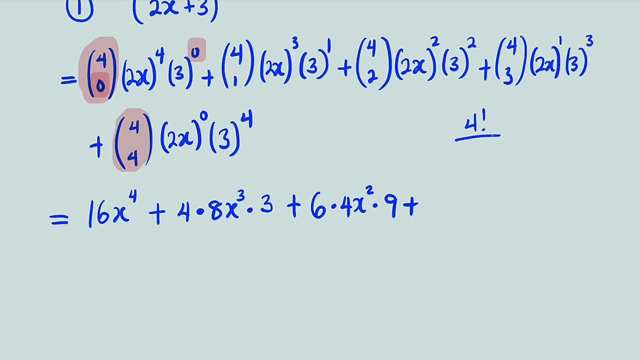 4 combination. 3 is 4 factorial divided by 4 minus 3 is 1 factorial, Then The 3 factorial. This is equal to 4 multiplied by 3 factorial, Divide by 1 times 3 factorial. So this will cancel this. 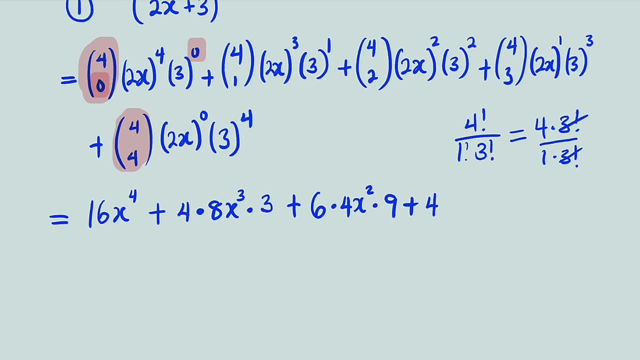 We have only 4.. So we have 4 here as 4 combination, 3. Then 2x to the power of 1 is 2x. Then 3 to the power of 3 is 27.. So we have 27.. 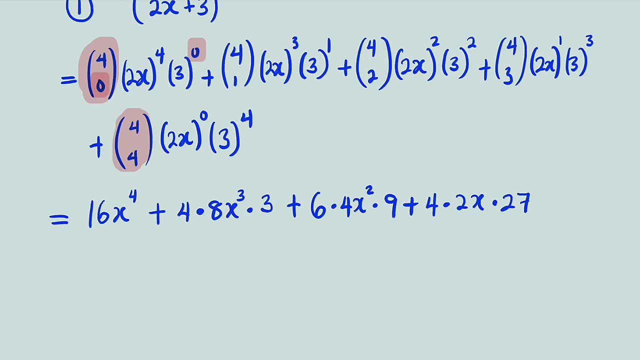 Then the last term. Already I told you, 4 combination, 4 is 7.. So we have only 2x to the power of 0, which is 1.. Multiply by 3 to the power of 4.. And 3 to the power of 4 is equal to 81.. 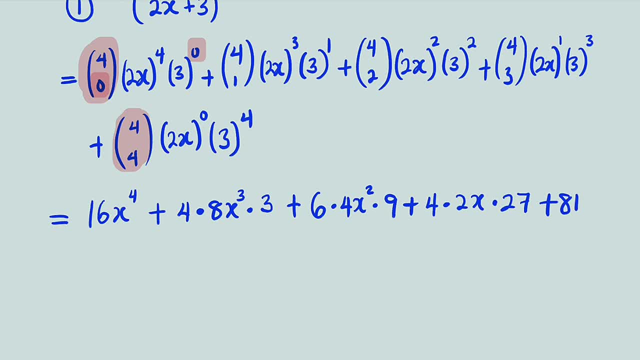 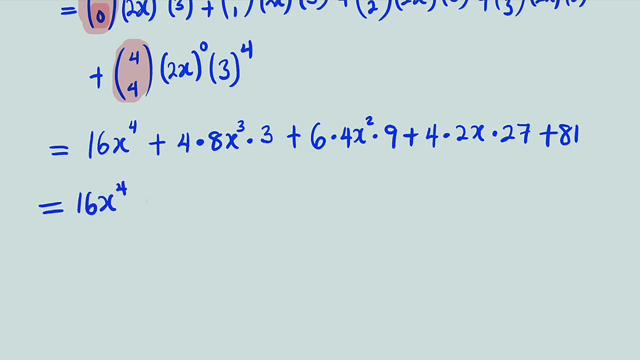 So the last term is just 81.. So let's further simplify this. Our first term is 16x to the power of 4, plus Now we have 4 times 8 times 3, which is 96.. So we have 96.. 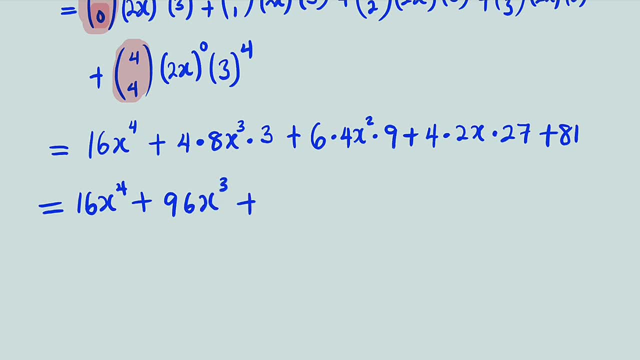 6x to the power of 3. plus Again, we have 6 times 4 times 9.. 6 times 4 is 24.. Then 24 times 9 is 216.. 216x to the power of 2.. 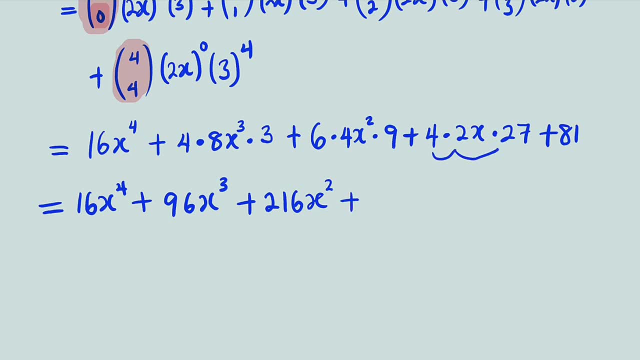 Then plus We have 4 times 2 times 27.. 4 times 2 is 8. And 8 times 27. So we have 9x to the power of 3 plus 9 will give us 216.. 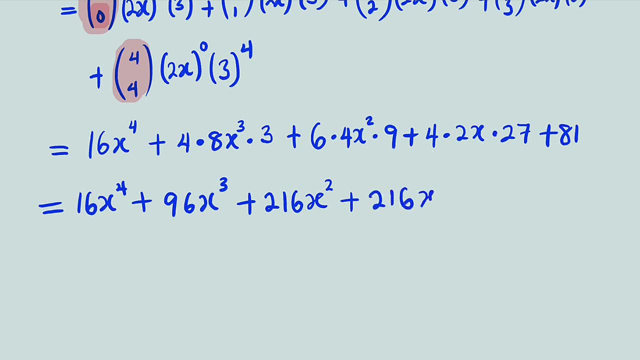 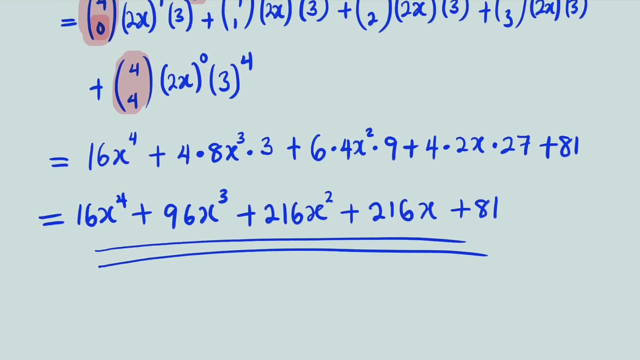 So we have 216x to the power of 1. And lastly, we have just 81. So this is just the expansion of 2x plus 3 to the power of 4.. Now let us take one more question. 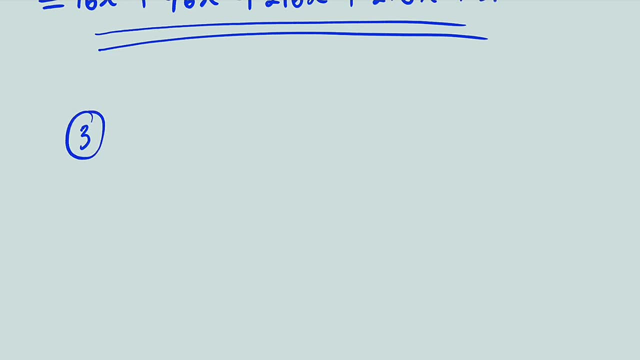 Let's take one more question. Suppose we wish to expand, maybe x minus 2y. Well, 1 minus x minus 2y plus 1 is. So let me take the previous one, Because our earlier one is equivalent to a zero. 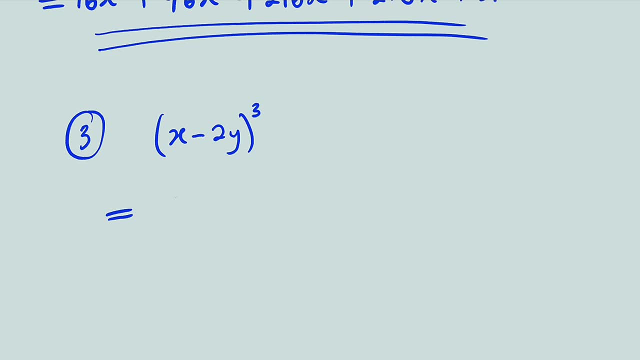 Let us take 1 minus x plus 3, which is this: get now 3 combination, 1 then a, which is x to the power of n minus 1. 3 minus 1 is 2. they multiply by the second term, 2, negative 2y, to the power of 1, then plus 3. 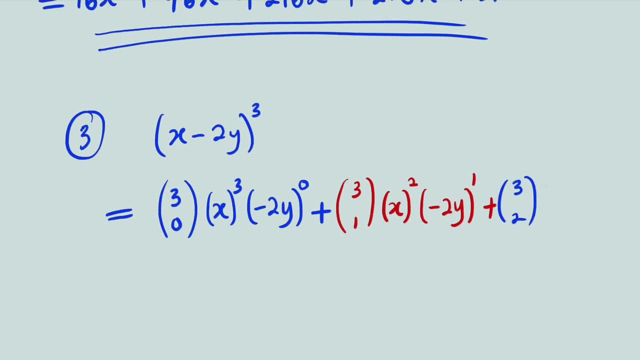 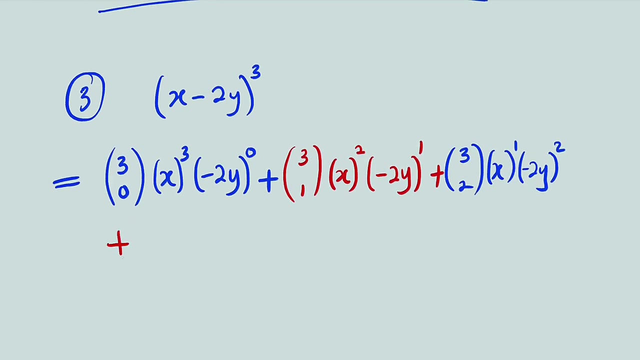 combination 2 X to the power of 3 minus 2 is 1, then negative 2y to the power of 2. then the last time we have 3 combination 3x raised to the power of 3 minus 3 is 0, the negative 2y to the power of. 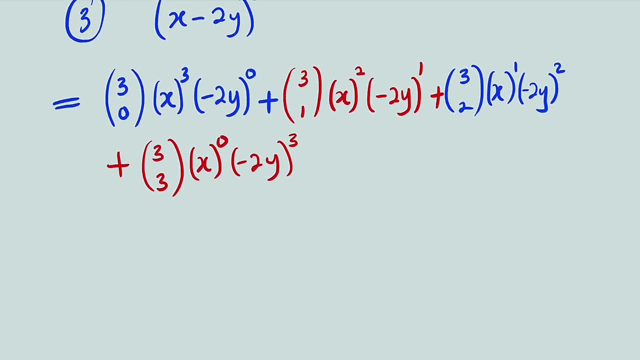 3. let's simplify this. remember I told you n combination 0 is 1, therefore 3 combination 0 is 1, and also n combination n is 1, so 3 combination 3 is 1. so from the first term, we know that this is equal to 1 as well, because any 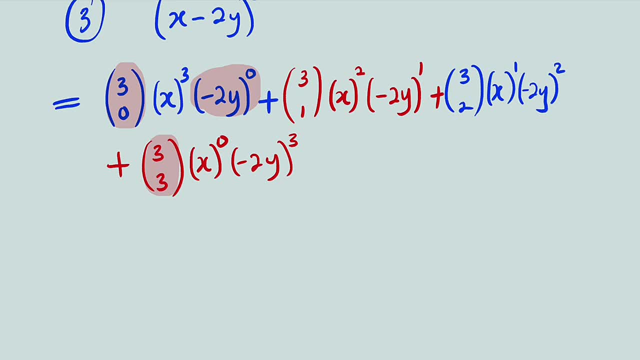 number to the power of 0 is equal to 1, except if that number is 0. so we only have X to the power of 3. so this is equal to X to the power of 3. then, plus, what we have here is 3 combination 1, which is the same thing as 3 factorial. 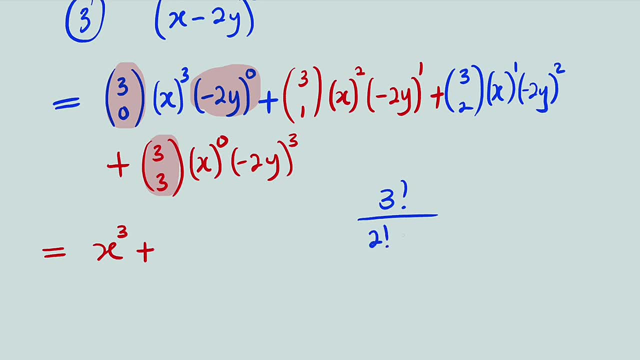 divided by 3 minus 1 is 2 factorial, then 1 factorial. if you simplify this, you have 3 multiplied by 2 factorial divided by 2 factorial times 1. 2 factorial will cancel 2 factorial. 3 divided by 1 is 3. 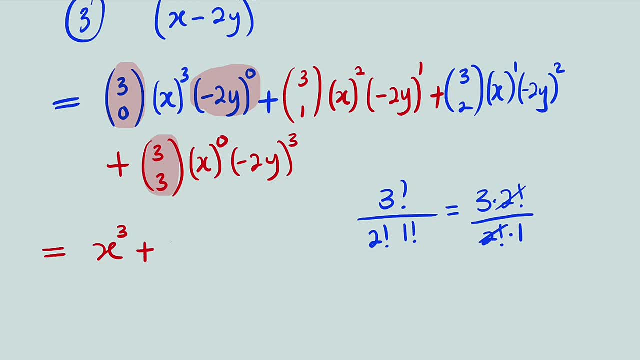 so 3 combination 1 is 3. this draw our attention to n. combination 1 is always equal to n. so 3 combination 1 is equal to 3. and we have, multiplied by X to the power of 2, is X squared multiplied by negative 2y to the power of 1 is: 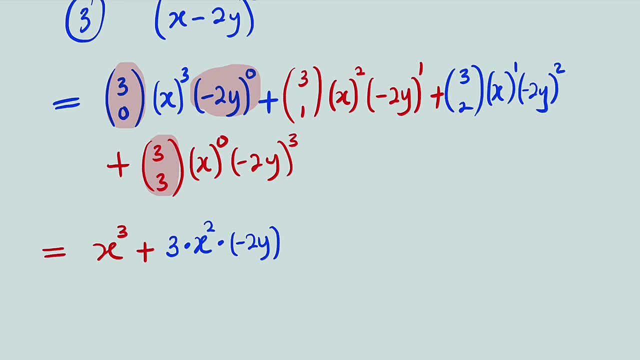 negative 2y. we take the next term, that is when we have three combination: 2, 3 factorial divided by 3 minus 2 is 1 factorial, then 2 factorial, which is equal to 3 multiplied by 2 factorial, divided by 1 times 2 factorial. this will cancel this, so we have 3 here. 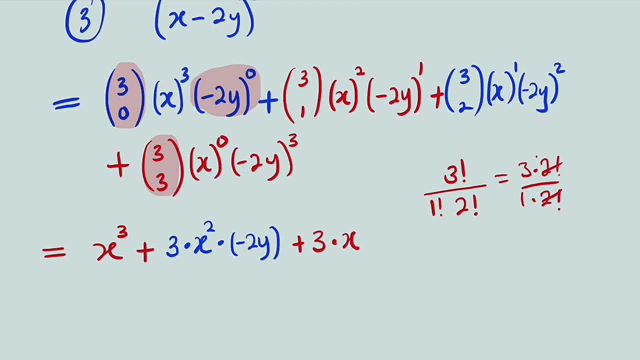 then X to the power of 1 is X. negative 2y to the power of 2 will give us 4 y squared. Then let us take the like term Already 3 combination: 3 is 1, x to the power of 0 is 1 also. so we only 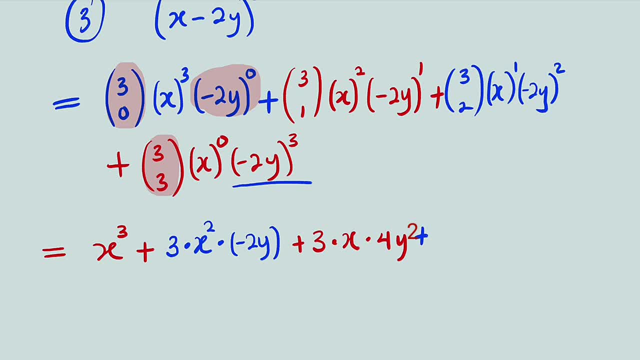 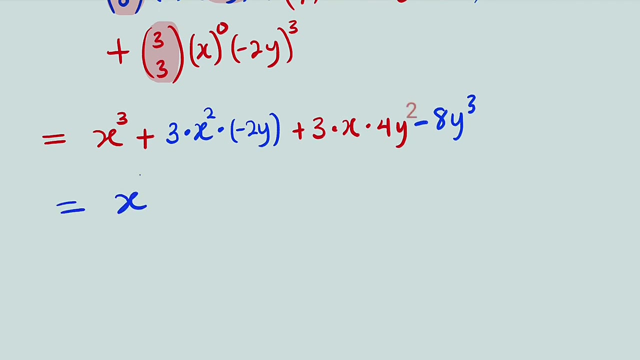 have this Negative 2y to the power of 3 will give us negative 8y to the power of 3, So we have negative 8y to the power of 3. Let's break it down for the last time. This is equal to x to the power of 3 plus. 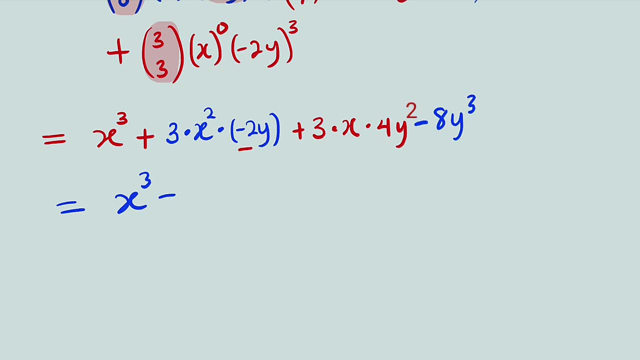 Ok, this will become negative because of this negative sign. We have 3 times this negative 2. that will give us negative 6, and we have x to the power of 2, then y to the power of 1.. We have plus sign: 3 times 4 is 12, so we have 12. 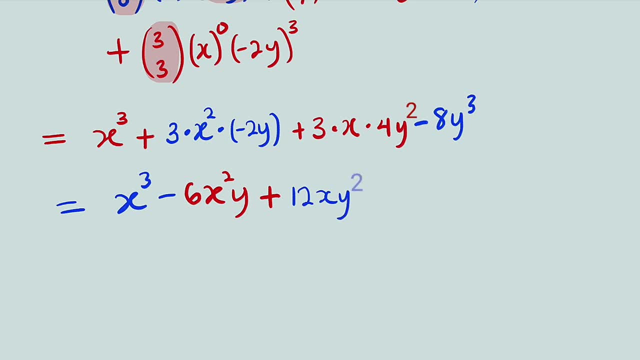 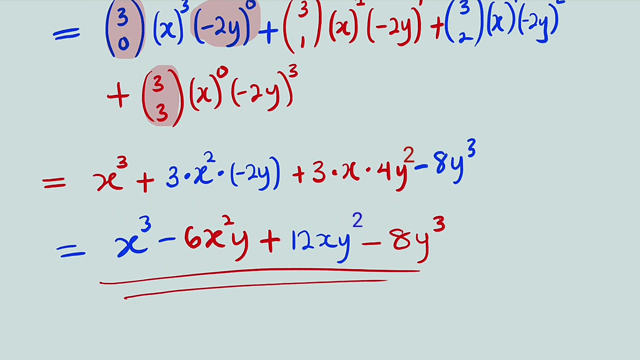 x, y and lastly, we have minus 8y to the third power. so this is just the expansion of x minus 2y to the power of 3, and this is all I have for you today. Thank you for watching. Do share to your learning colleagues and don't forget to. 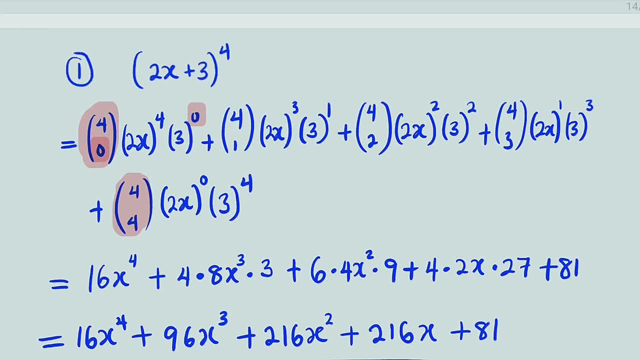 subscribe to my youtube channel for more exciting videos. Subsequently, we are going to look on to how to find the n-term of binomial expansion using this combination. Bye, bye. Subtitles by the Amaraorg community.